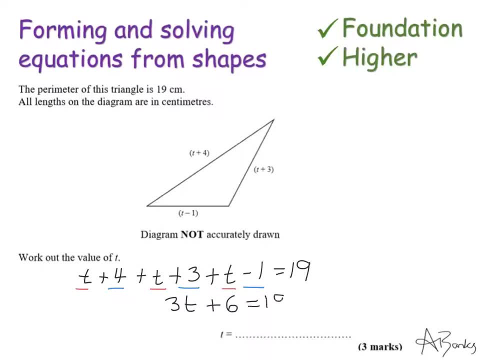 So 3t add 6 is 19.. So now I can solve this equation. I'm just going to do that up here. So 3t add 6 equals 19.. So I'm going to take away 6 from both sides. 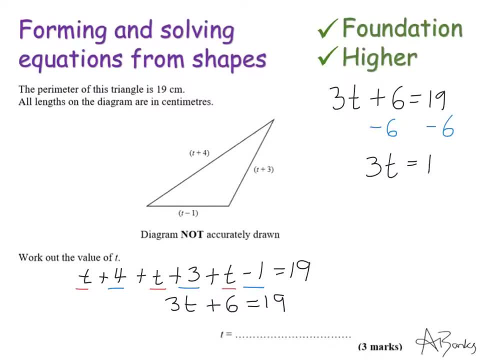 That'll give me 3t equals 13. And then divide both sides by 3.. Now I know that I can't divide 13 by 3 perfectly. My answer's not going to be an integer, So I can just write 13 over 3 as a fraction. 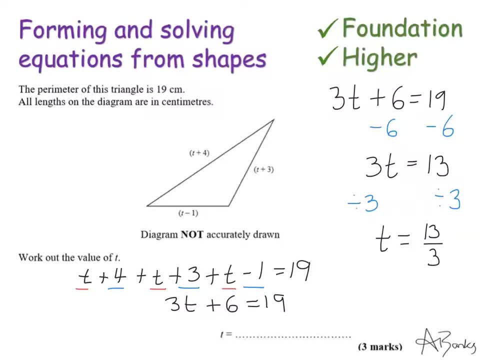 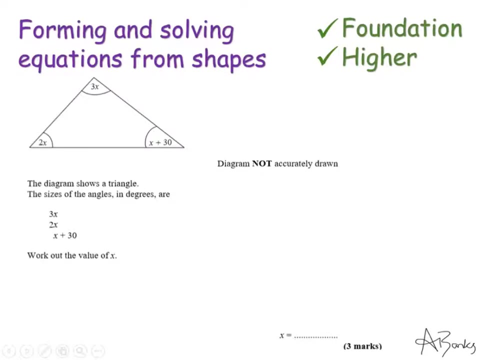 And that's it. that's fine to leave my answer like that. I could convert it into a mixed number, so that will be 4 and a third, but either one of these answers is fine, and that is my value of t. Here's a slightly different example for us to look at. This question says the: 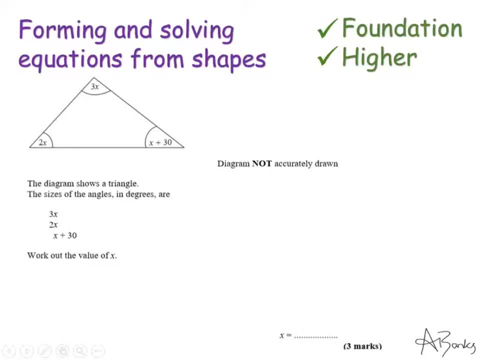 diagram shows a triangle. the sizes of the angles in degrees are 3x, 2x and x. add 30. Work out the value of x. So they've not really given me any information in the question here. that will let me form an equation. I've got the size of the angles, but that's it This. 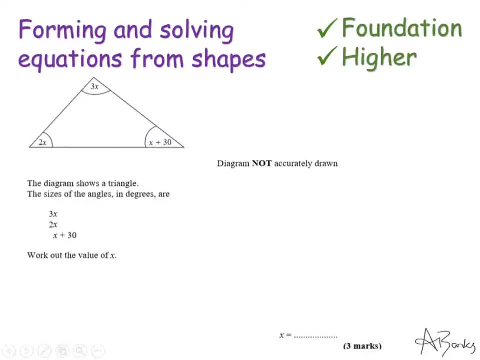 is because they're expecting you to know that the angles in a triangle add up to 180.. So the equation I can write is that the three angles, so the 3x, add the 2x, add x, add 30, add 80, equals 180.. So that's my first step, So I can simplify this just like before. So 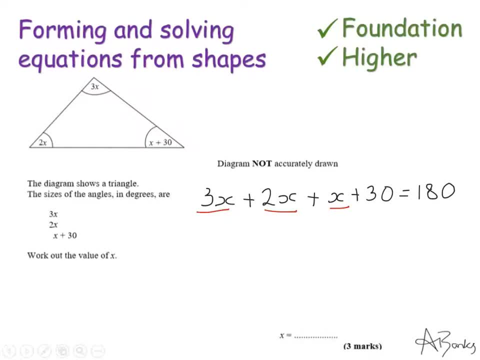 I've got 3x, 2x and 1x, So all together I have 6x, and I also have my plus 30. So plus 30 equals 180.. And I can solve this equation. So subtract 30 from both sides, I've got. 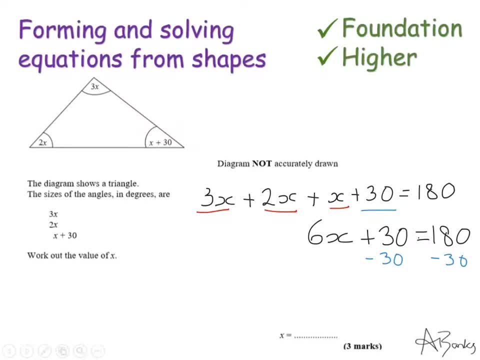 6x, I have 6x equals 150.. And then divide by 6. I get that x equals 25.. And that's my answer. It's worth noting here that on both of these examples I've just completed the. 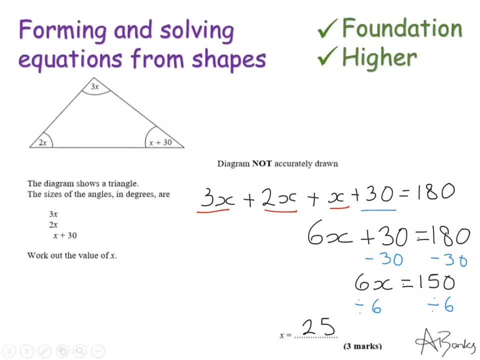 question could be: work out the value of x, So I've got 6x, 2x and 1x, So I've got 6x and 1x, So I can work out the value of the largest angle or work out the value of the. 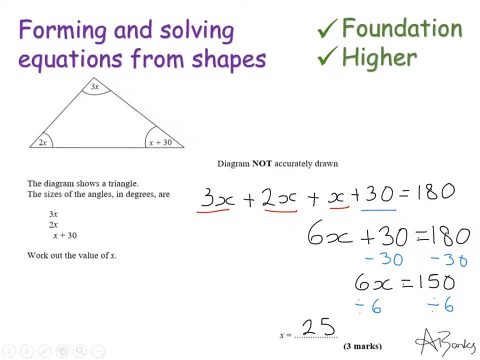 smallest side, And all this would mean doing is substituting this value here, this 25, back into these three angles. So let's say the question was: work out the size of the largest angle. Well, 3x would be 3 times 25,, which is 75.. 2x would be 2 times 25,, which 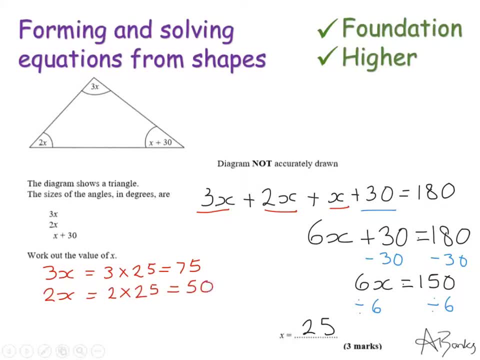 equals 50. And x add 30 would be 25. add 30,, which would be 55. So the size of the largest angle would be the 75 here. This is also a great way of checking that I've done my answer. 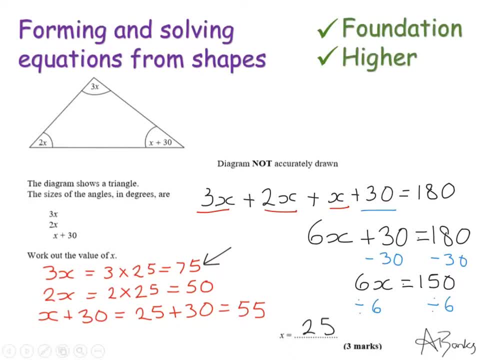 right. I said that the angles in a triangle add up to 180 degrees. So if I've done this right, 75 add 50 add 55 should be 180.. And if I add them together I know it is 180.. 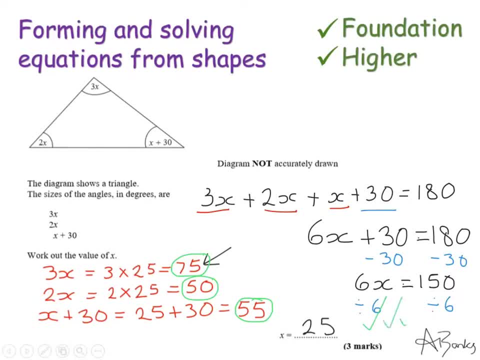 So I've done this question right and I've banked these three marks In question one. it might have been difficult on a non-calculator paper for me to spend the time working out what the length of the three sides were, because my answer was a complicated fraction. I could. have done, but it might have been difficult. So I've done this question right and I've spent the time working out what the length of the three sides were, because my answer was a complicated fraction. I could have done, but it might have been difficult, So I've 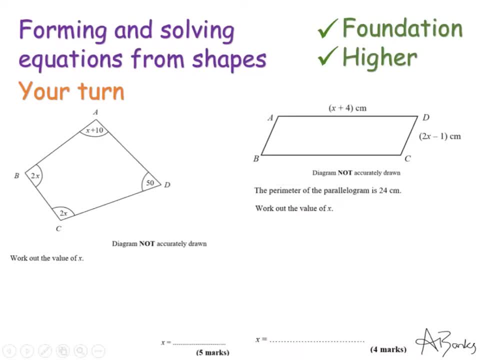 done this question right and I've spent the time working out what the length of the three sides were, because my answer was a complicated fraction. I could have done, but it might not be worth the time. Here are two questions for you to try. The first one is the angles. 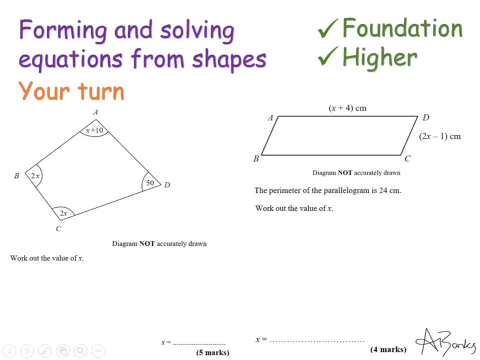 in a quadrilateral, and the second one is another perimeter question. If you pause the video now, then play when you're ready to see the solutions. So here are the two solutions You should have got for the first one that x is 60. And if you're looking green, I've